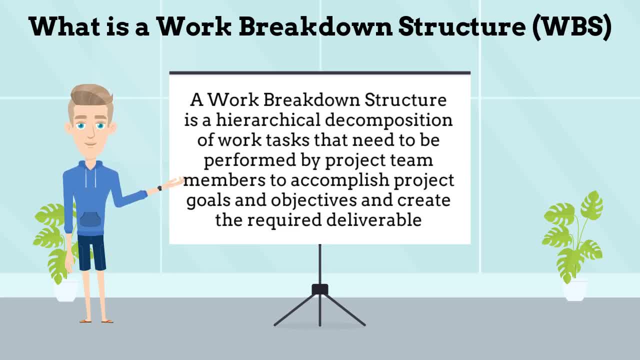 The WBS displays and defines the product to be developed and produced. It relates the elements of work to be accomplished to each other and to the final product. In other words, the WBS is an organized method to break down a product into sub-products at lower levels of detail. 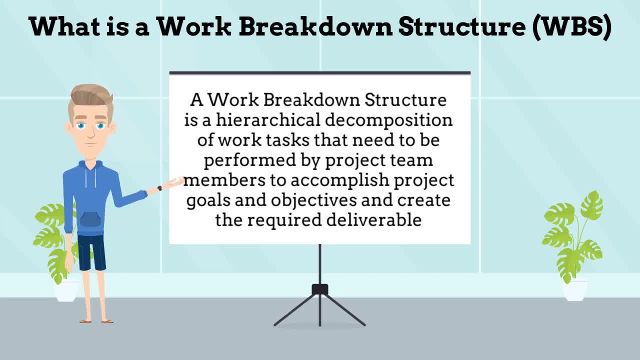 The WBS is used for planning, cost estimating, execution and control. Per the definition, a Work Breakdown Structure is a hierarchical decomposition of work tasks that need to be performed by project team members to accomplish project goals and objectives and create the required deliverable. 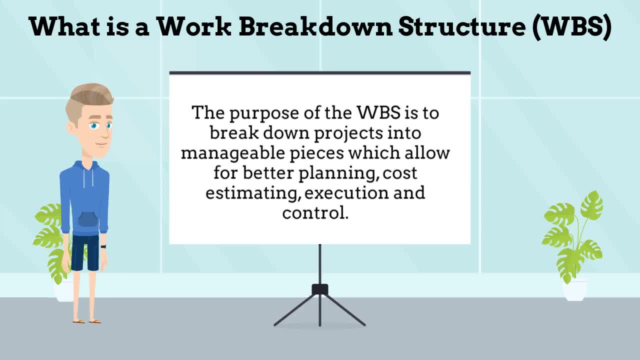 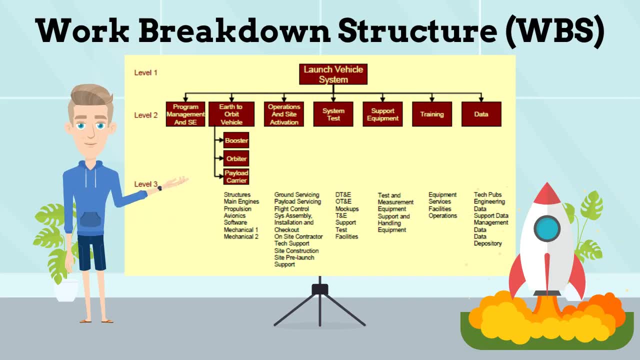 The purpose of the WBS is to break down projects into manageable pieces which allow for better planning, cost estimating, execution and control. Here is an example of the Work Breakdown Structure from a rocket program. This WBS shows the first three levels of the rocket project. 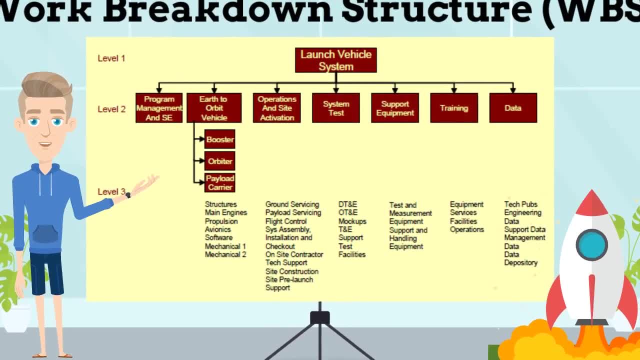 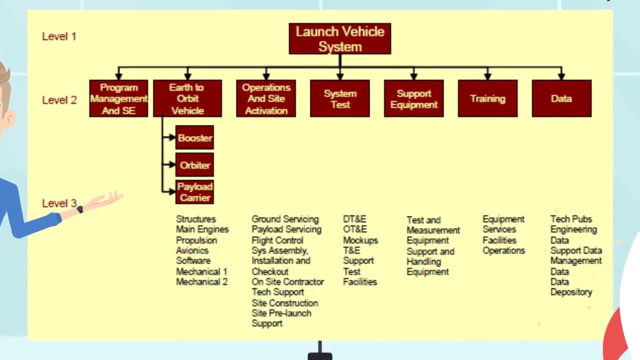 The government or customer program manager, with the support of systems engineering, usually develops the first three levels of the program WBS. They then provide it to the contractors who further define the WBS into more discrete elements. A completed WBS can have 10 or more levels. 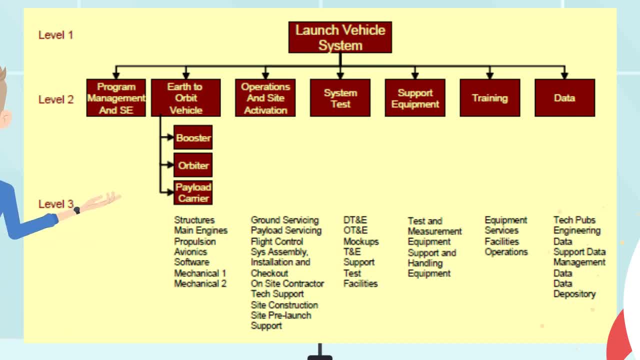 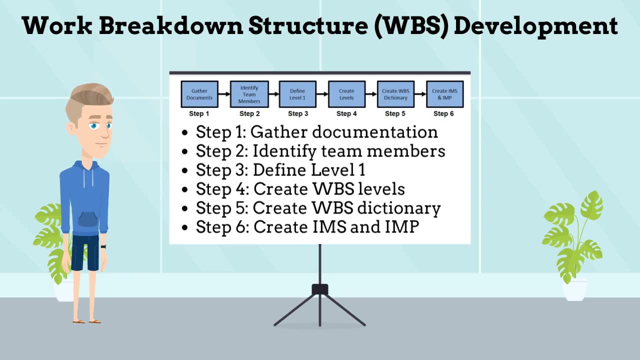 The first three Work Breakdown Structure levels are organized as Level 1, Overall System. Level 2, Major Elements. Level 3, Subordinate Components. The process of developing a WBS is straightforward but requires preparation and a clear understanding of what is required to be accomplished on a project. 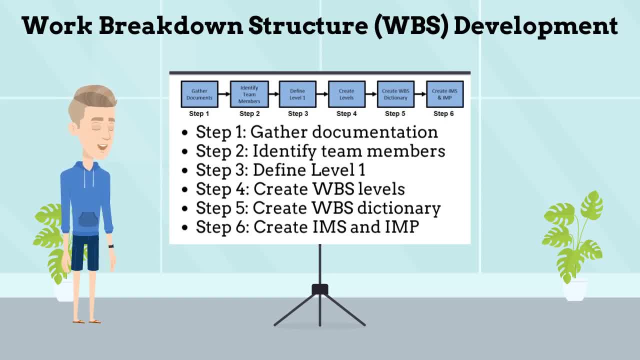 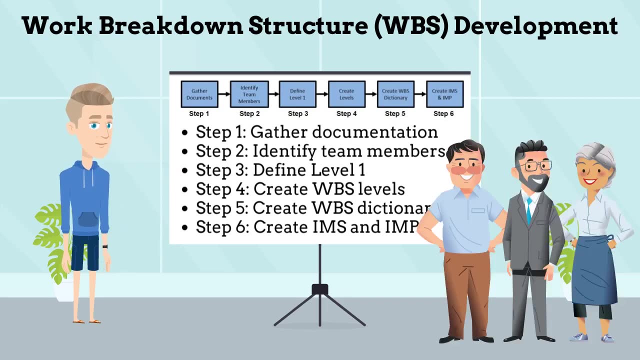 There are six steps associated with the development of a WBS. Step 1, Gather Main Documentation. Step 2, Identify the Project Goals and Objectives. To do this, gather the Project Charter, Scope, Objectives and any Requirements. Step 2, Identify your Main Team Members. 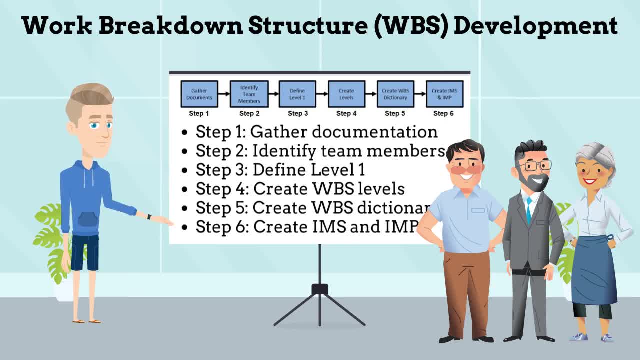 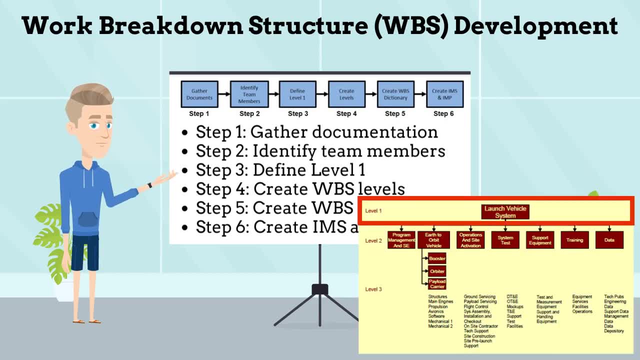 A WBS cannot be built in a vacuum. It takes a team of specialized people to know how to break their sections down into discrete elements. Step 3, Define WBS Level 1. This level is a summary of the deliverable that must be met to satisfy the project scope.